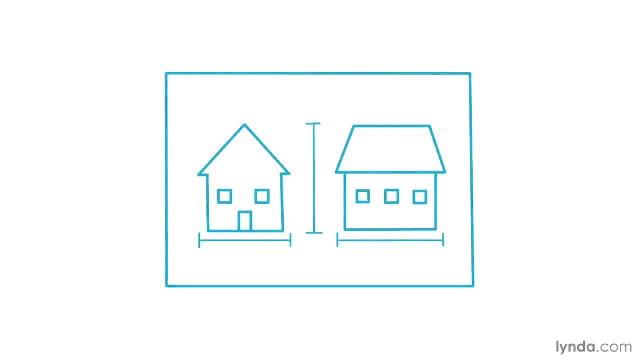 Now, when you build a house, you need blueprints, materials, people to put it all together and someone who wants to test it. This will manage the overall project. Before you start, you generally apply for permits and then you'll have some inspections along the way. 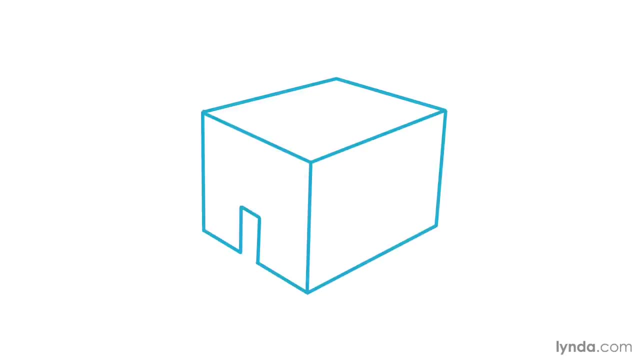 Let's say we have our basic framing for our house and an electrician is starting to run wires that ultimately will be concealed within the walls. Once the wiring is in place, an inspector will generally want to schedule a time to inspect the work. 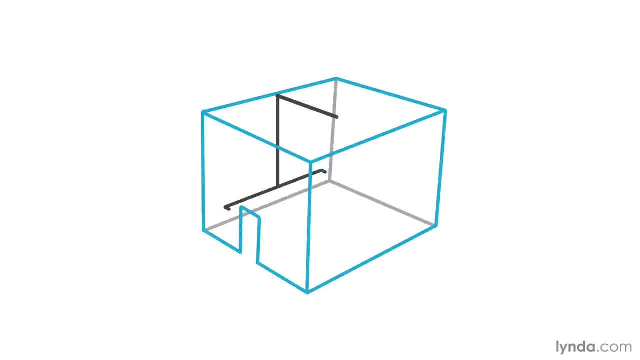 Now, some people find this inconvenient and unnecessary, as their perception is that it will slow down progress. but that's not really the case. If you were to move forward without inspecting to ensure that there were no problems, let's just think about what that might look like. First, someone would likely add insulation within your walls. Then new sheetrock would be installed over the insulation and wiring. Then there's usually tape applied to the seams in the sheetrock. Next, a texture may be applied to the walls. 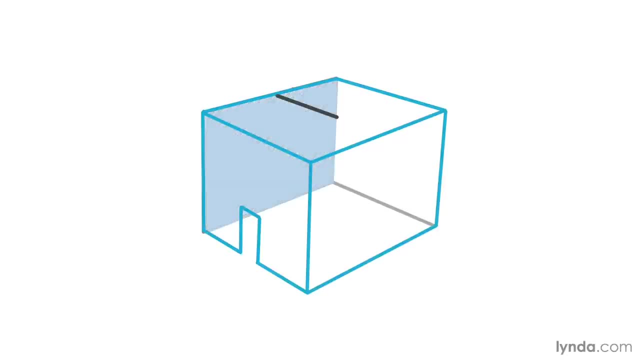 Eventually they'll be primed and painted. The further along in the process you get, the harder and more expensive it will be to go back and fix a problem that occurred at an earlier step. Keep in mind you aren't just paying for the issue you discovered. 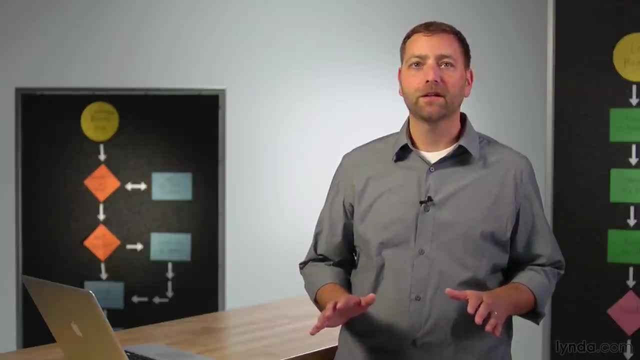 It's not just a basic materials cost. There's also a human factor in the labor involved and some steps may be owned by different individuals, which can make it more costly. If you had inspected your wiring before anything else was done and found a problem, 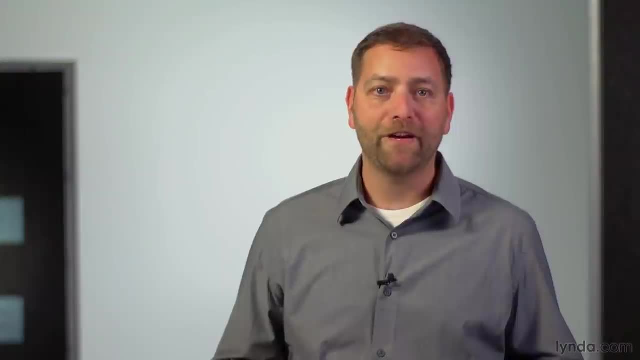 you would have only a single individual who would have had to fix a single problem and nothing else in the series of steps would have been done. In actuality, you would have saved quite a bit of time and money If you discover an issue after every step has been completed. 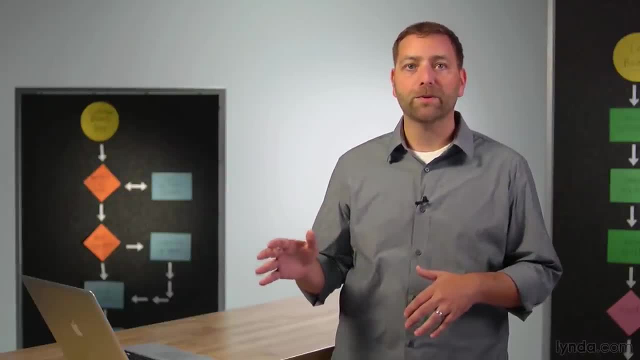 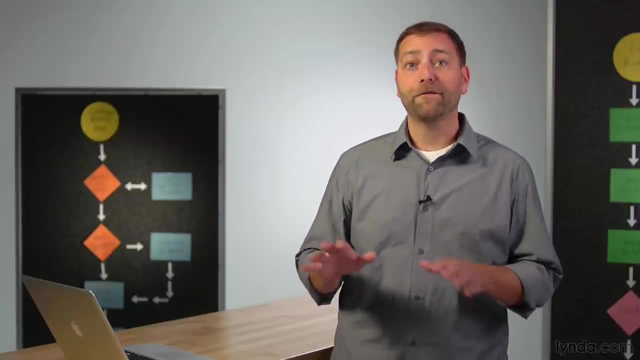 there can be a lot that has to be undone in order to address it. This philosophy holds true with software, and it's one that should be embraced. Bugs that are found and fixed early are less costly to address If you've been thinking about quality throughout the development process. 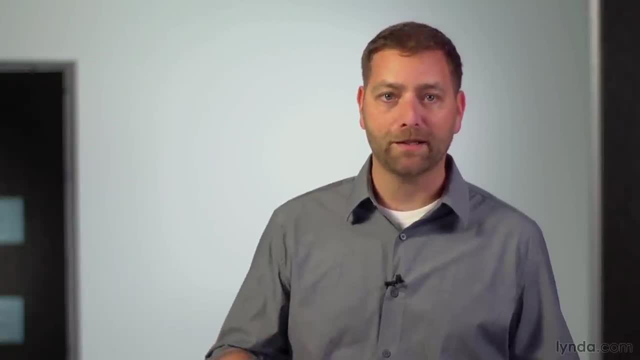 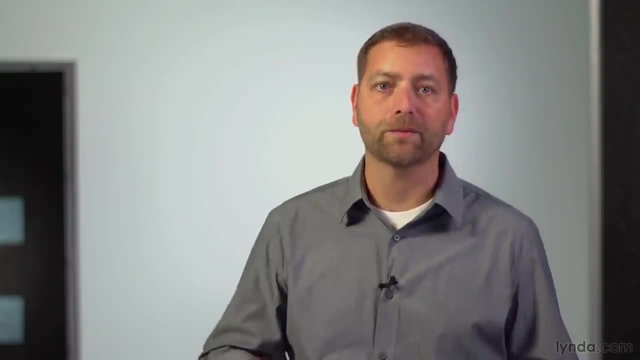 you're able to deploy the right systems at the right time. It's not about delaying a project, Slowing down progress or calling out a single developer who might have caused an issue. It's more a practice of operational efficiency. Not only are you trying to get features implemented,